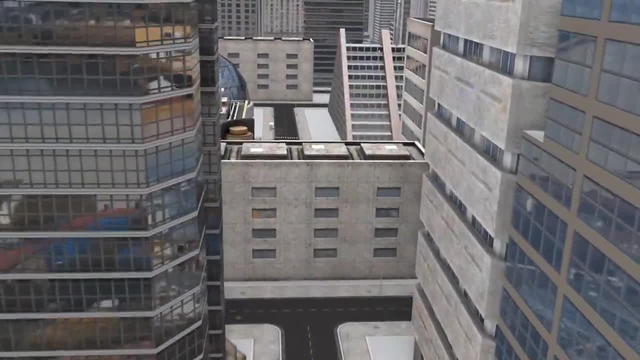 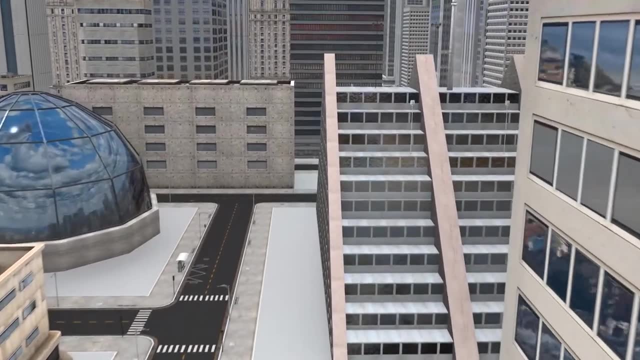 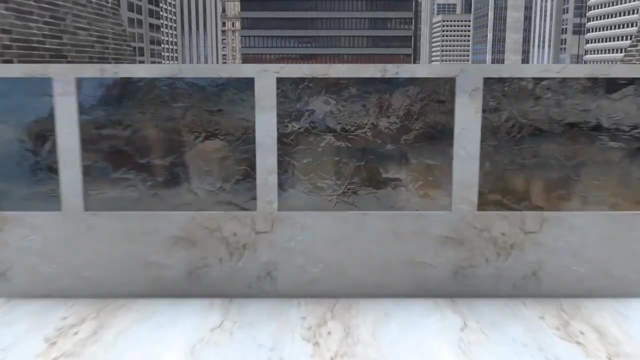 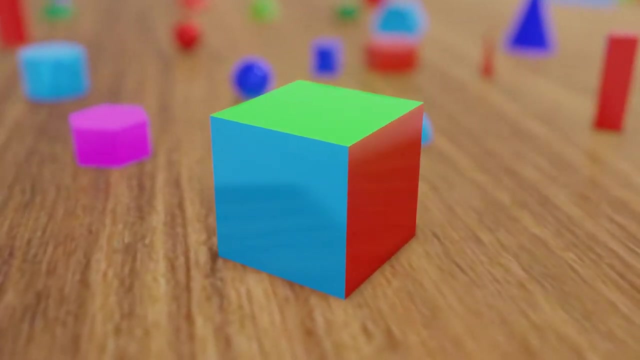 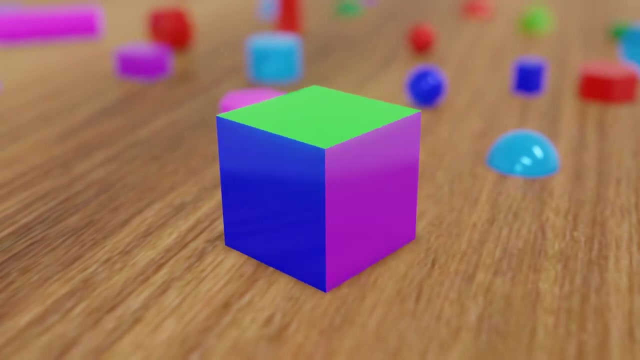 We will learn how to visualize solid objects and have a look at how they appear when viewed from different sides. Let's look at this cube. It is a three-dimensional object as it occupies space. Let us observe this cube from different directions. We will look at the top view. 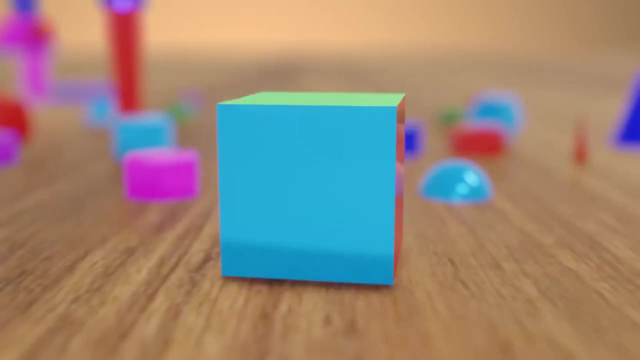 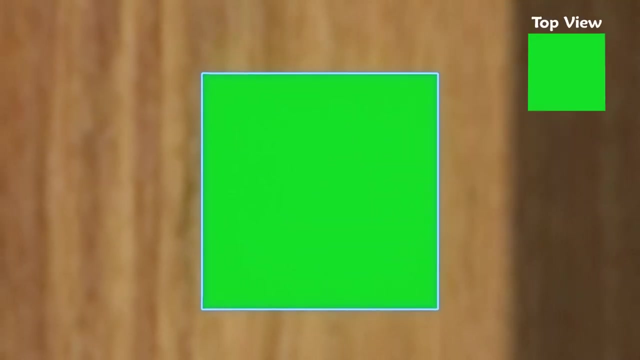 the front view and the side view. How will this cube look when you are viewing it from the top? All we would see is the top face, which is a square. The top view of the cube is a square. Let's bring it back to the original position. How would the cube look if we view it from the 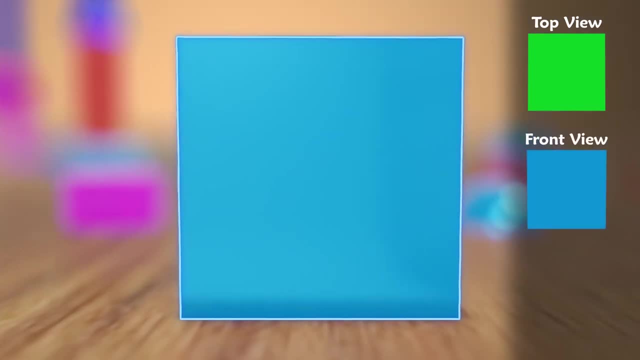 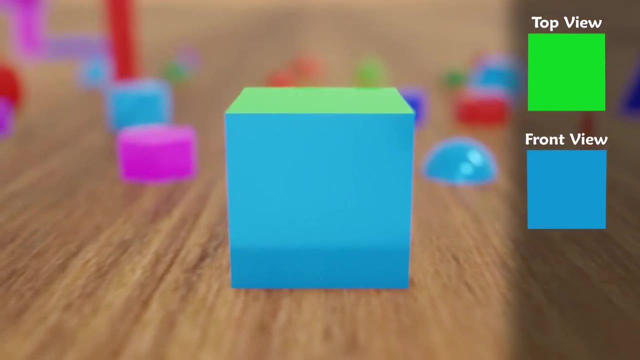 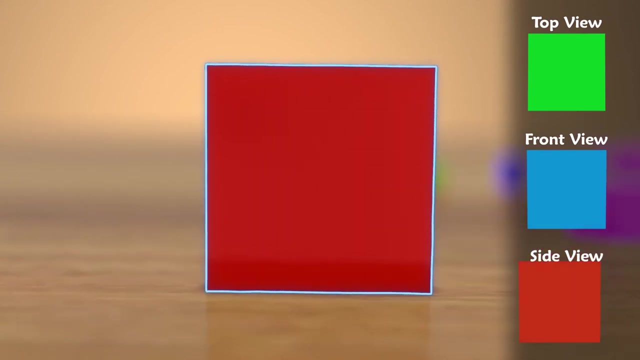 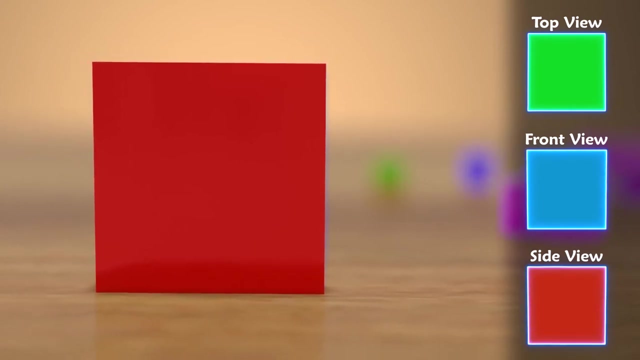 front, We would just see the front face, which is also a square. Let's bring it back to the original position. How would it look if we view it from the right side? It's a square again. If we observe cube from the top view, front view and the side view, we will always see a square. This involves: 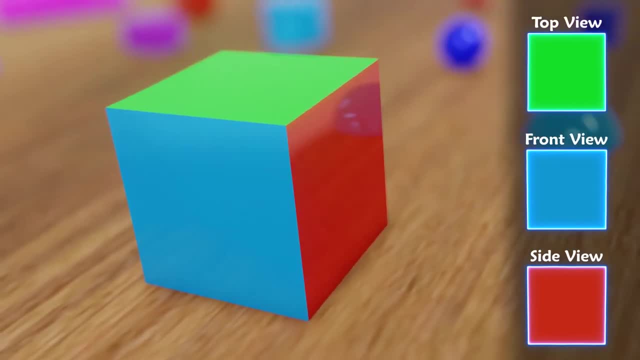 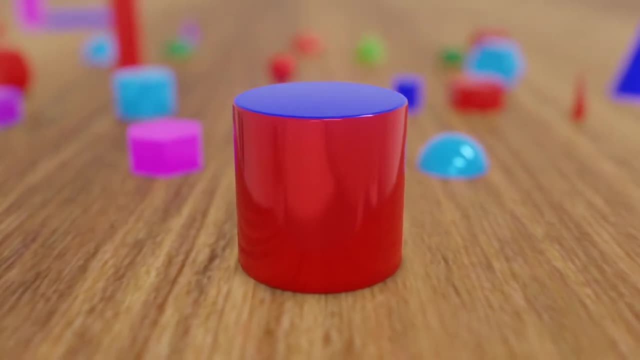 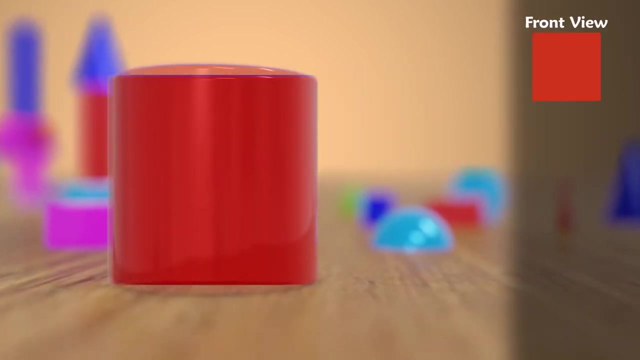 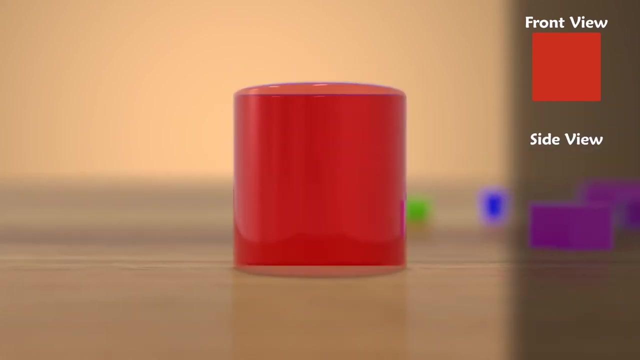 a bit of imagination and we will try it out with different shapes. Let's consider a cylinder. How would a cylinder look if we look at it from the front? The front view would be a rectangle. Now let us observe the cylinder from the side, That is, let's have the side view. It again has the 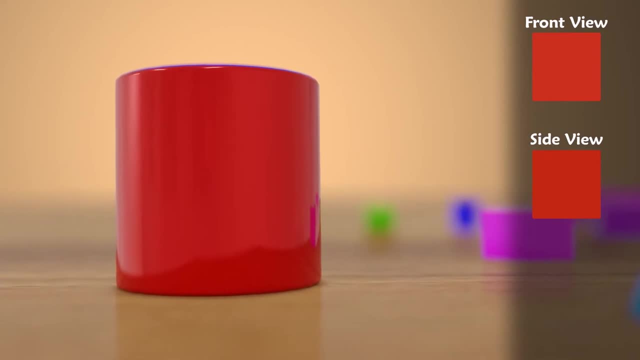 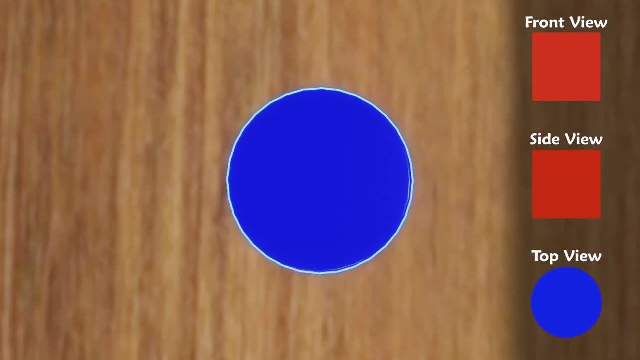 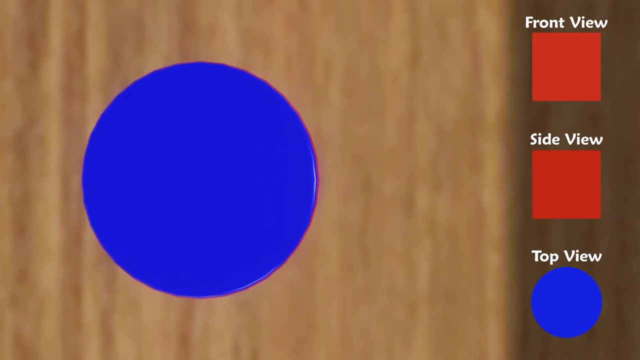 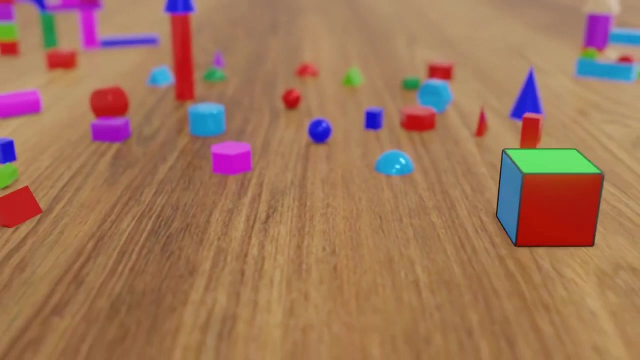 shape of the rectangle. Will it be rectangle again if viewed from the top? No, The top view of the cylinder is not a rectangle, but it is a circle. So imagining the views was pretty easy here. How about we making it more exciting? Let us place the eight cubes next to each other in this manner We